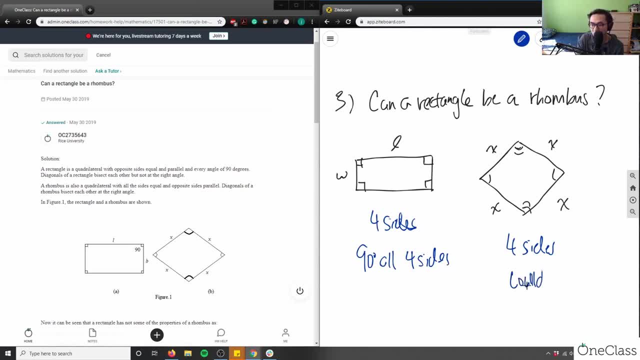 So we can say: could also, could also be 90 degrees. And then we have here. we have here the length, The length of the sides. right, We care about the length of the sides In a rectangle. if the length was the same, it would just be a square, right. 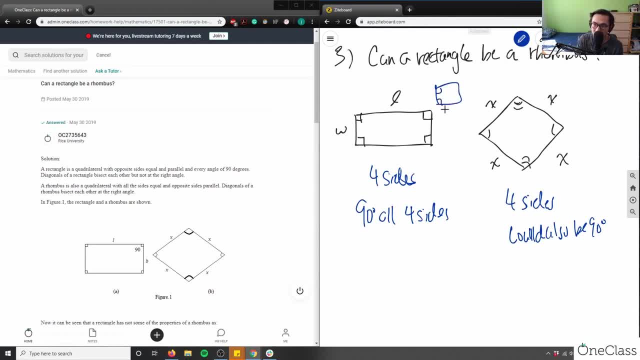 Remember a square here has has has right angles on all four sides And the, the length and the width are the same right. So length is, I can say that this is X and this is also X, But in a rectangle the length has to be greater than the width. 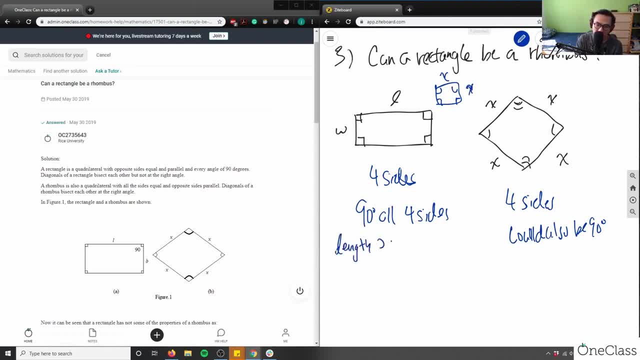 So I have to say length is greater than the width for our, our length of the sides And then the rhombus. all sides are equal, So these. so I just compared three kind of properties of a rectangle and a rhombus. 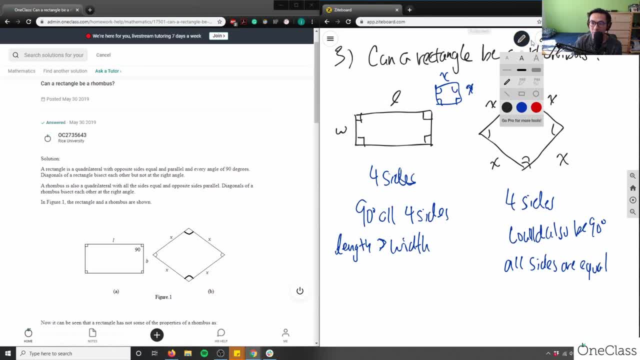 So in this case, let's look at, so let's look at our our chart. here We have four sides, both of our four sides. that's good. So let me do that in red, that's good. 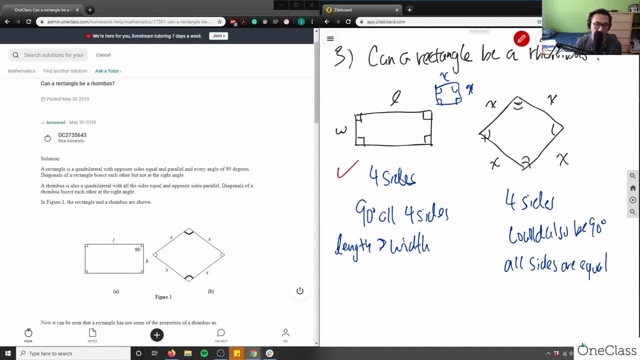 So side length, so number of sides, is perfect. So they're both quadrilateral, so which are perfectly fine: 90 degrees on all four sides. This could also be 90 degrees for a side. An example could be that these four sides could, or four angles. 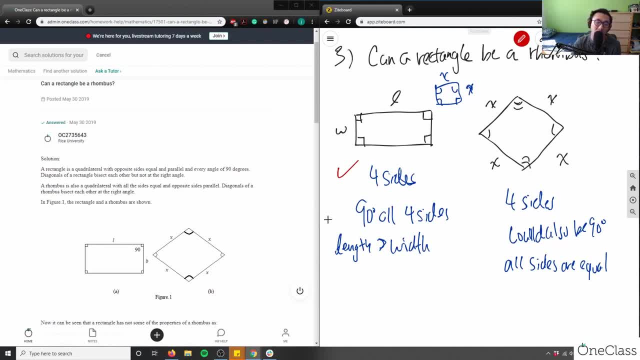 It could be 90 degrees, but they don't have to be. So this technically is, is also satisfied, depending on what the angle is. depending on if I differ the differ the angles. And then here it says length has to be greater than the width. 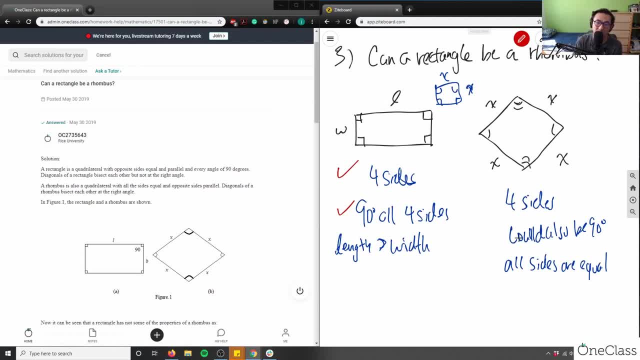 but in rhombus, in a rhombus, all sides are equal. So this case it does not meet the, does not meet the requirement right, Because if all sides are equal, if all sides are equal, then I would go, I would get. this is the property of a square right. 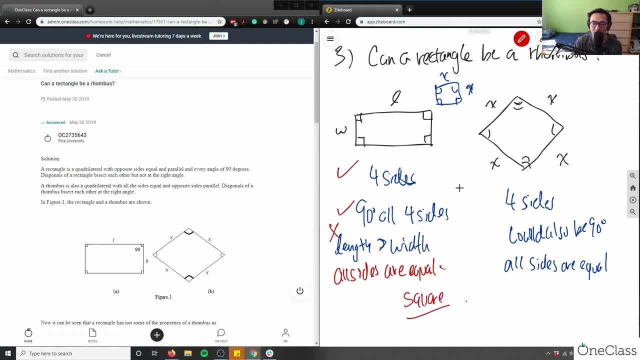 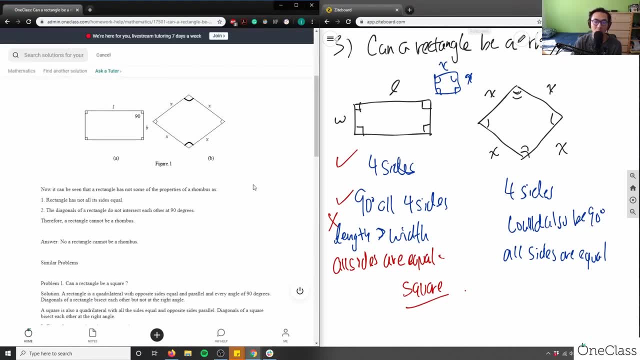 Which is not a rectangle, which means I'm fulfilling step one, step two, but step three. the criteria is not being met here. So if the step three is not being met here, the rectangle cannot be a rhombus. 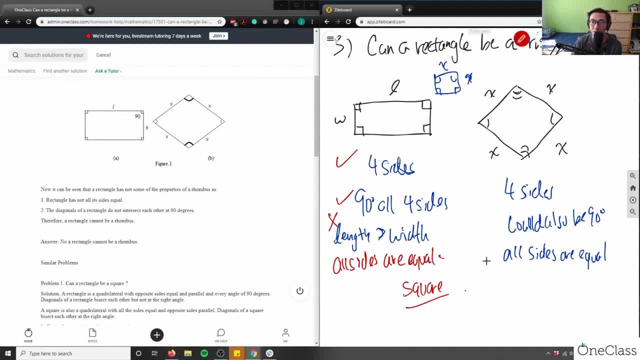 So in this case- that's going to be my answer here- Rectangle cannot be a rhombus, Cannot be a rhombus Because of this, this, this, this, this kind of criteria. here the all sides are equal. 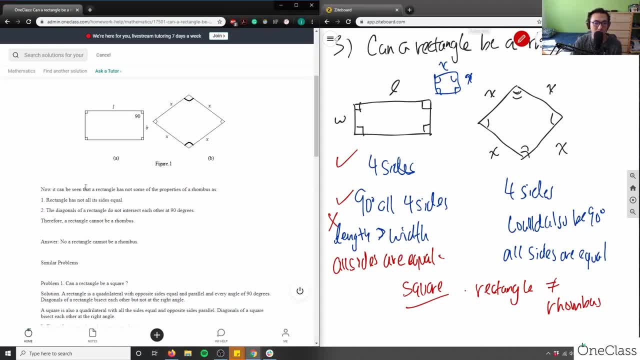 It's not because all sides cannot be equal to each other. So the result I like. so let's see, Let's do this here, So now it can. now it is seen that rectangles has not some of the properties. 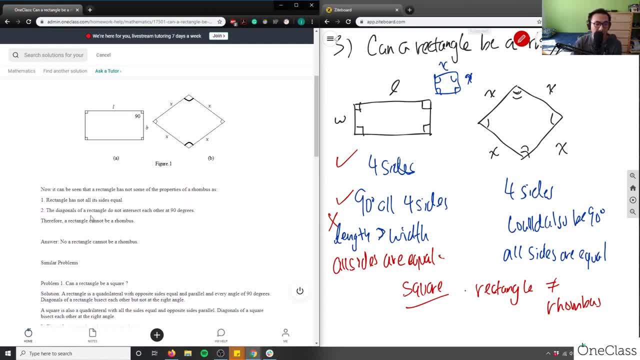 Rectangle has not all sides. That's what we proved. And the diagonals of a rectangle do not intersect each other at 90 degrees, And that's actually proof. That's also correct, right? So if I drew a diagonal between here and here and here and here, 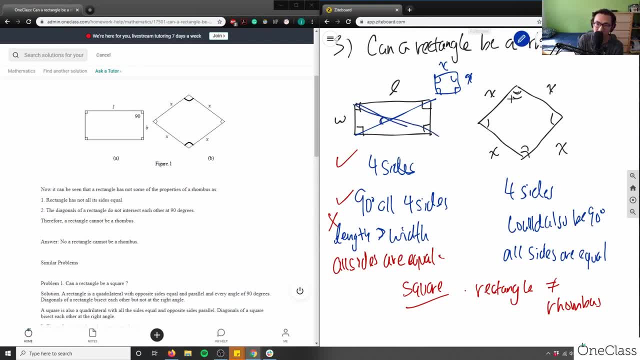 sorry, this is a really bad diagonal. They don't intersect each other at 90 degrees. These are not 90 degree angles here, But in this case, if I drew a diagonal from here to here and here to here, this is a right angle here. 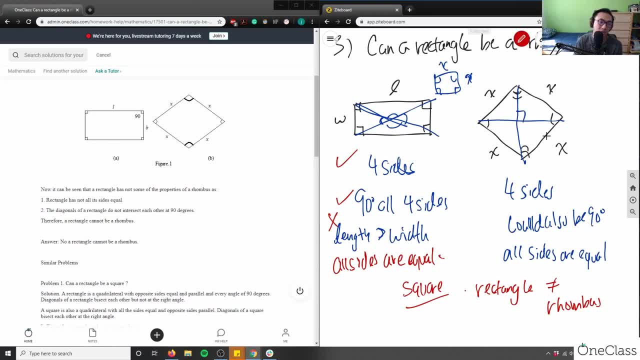 So in this case, again because of the diagonal, it's also not a rectangle here. So diagonal is or diagonals. sorry, diagonals are not 90 degrees. That's also another property that I didn't actually talk about. 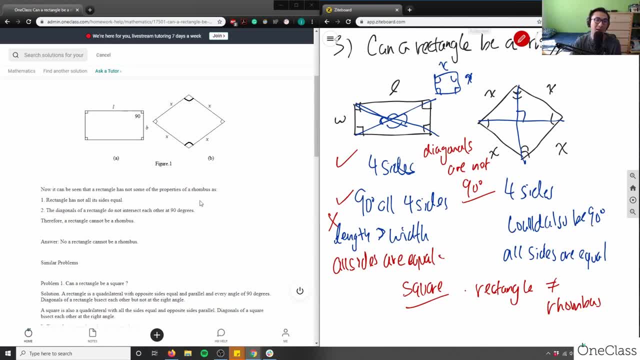 but they use that to support their argument. Totally fine, That's even better. I actually had a better answer than I did, Because I only proved it by sides, but they proved it by diagonals as well. So therefore, rectangle is not a rhombus. 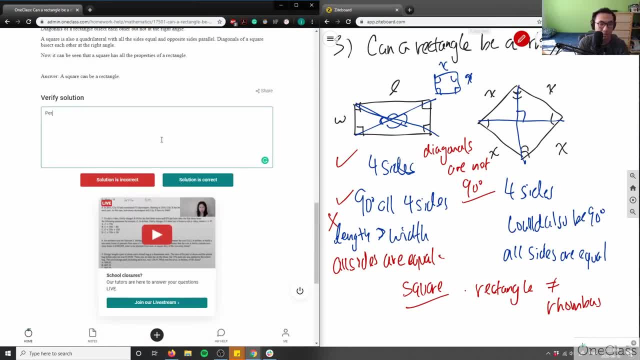 This here is a perfect solution. So I'm going to say here: perfect solution, Solution and great analysis. So solution is correct. 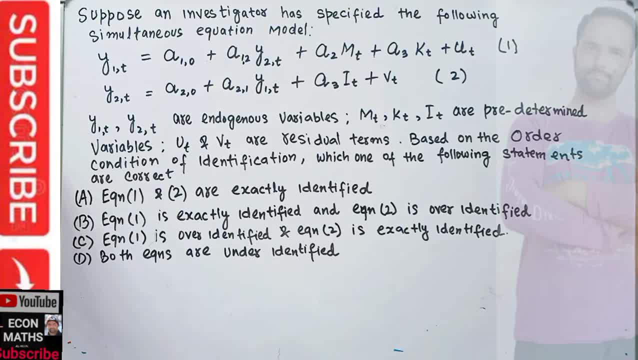 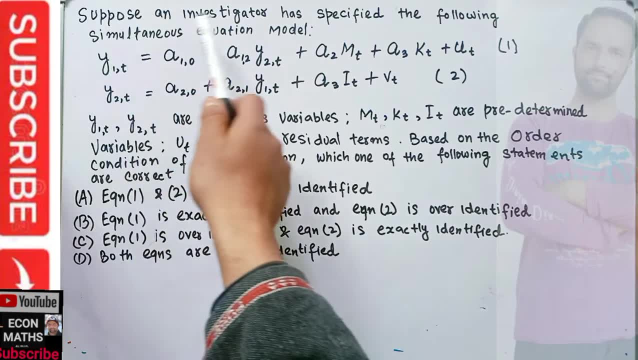 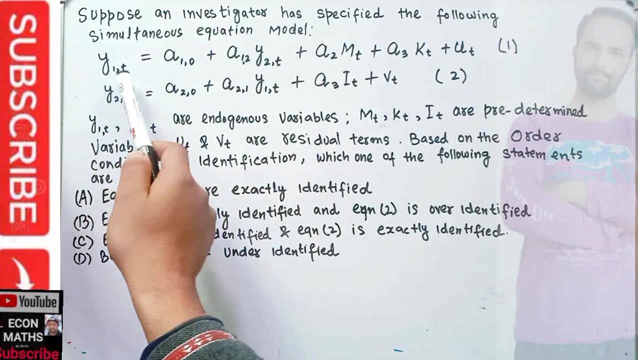 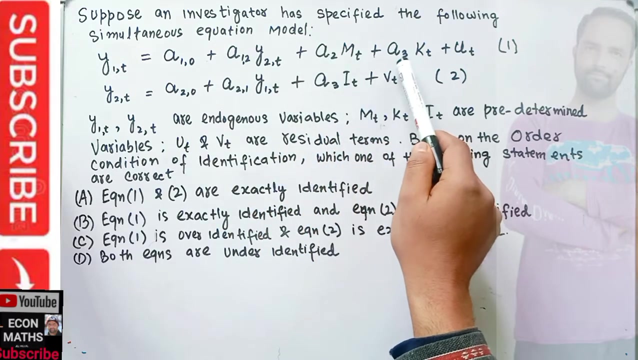 In this video we will try to solve another question that was asked in Gate Economics paper of 2022.. The question is related to identification problem. The question is like this: Suppose an investigator has specified following simultaneous equation model. We have this simultaneous equation model where y1t is equal to alpha 1, 0 plus alpha 1, 2, y2t plus a2, mt plus a3, kt plus ut. This is our equation. first and second equation is y2t.